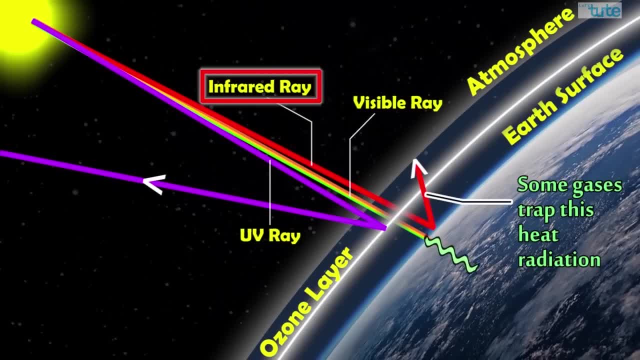 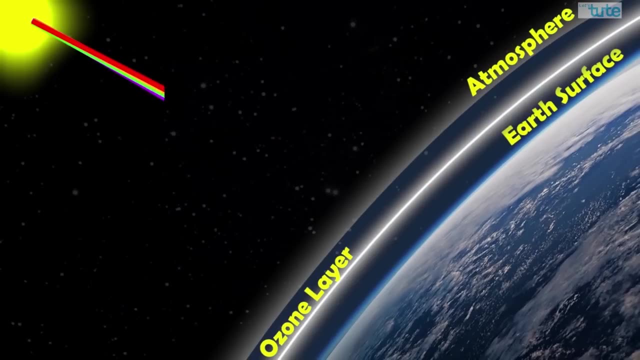 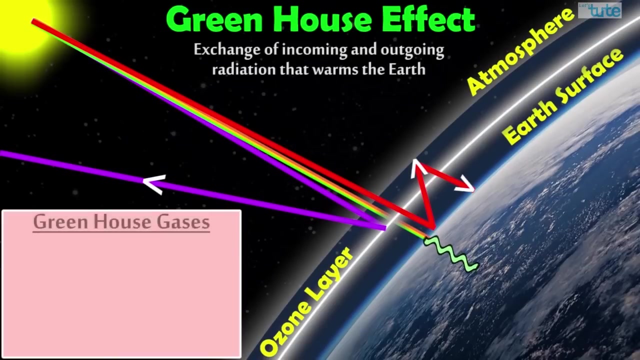 But some gases in the atmosphere traps this heat radiation And re-emits it to the surface, which leads to heating up of the environment. This exchange of incoming and outgoing radiation that warms the earth is referred as the greenhouse effect, And the gases involved in this are called greenhouse gases, which mainly includes carbon. 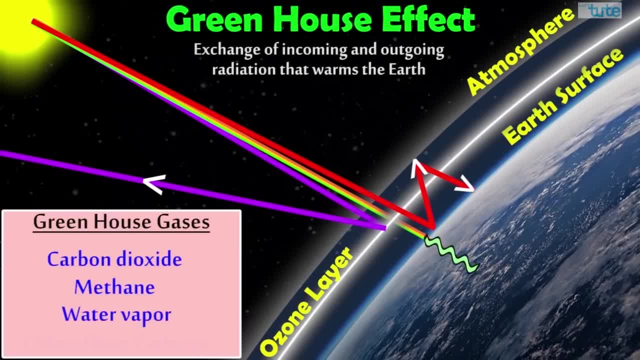 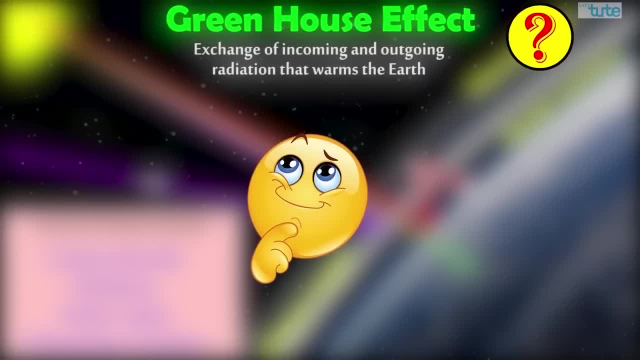 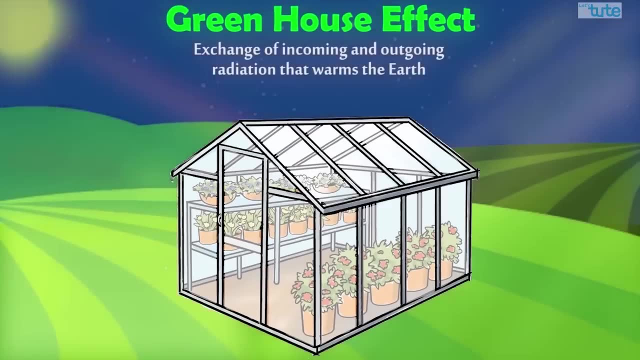 dioxide, methane, water vapour, chlorofluorocarbons, etc. Friends, but are you not wondering why it is called greenhouse effect? Is it something to do with the greenhouse? If you said yes, you are thinking in the right way. 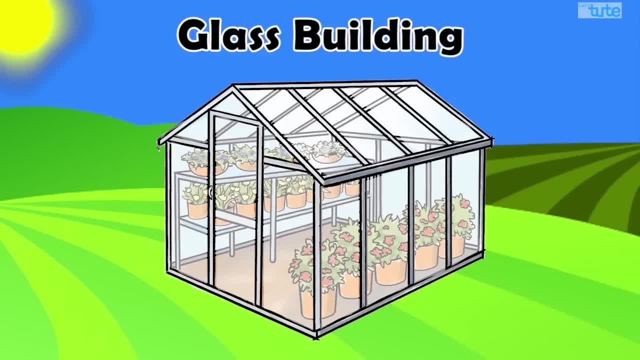 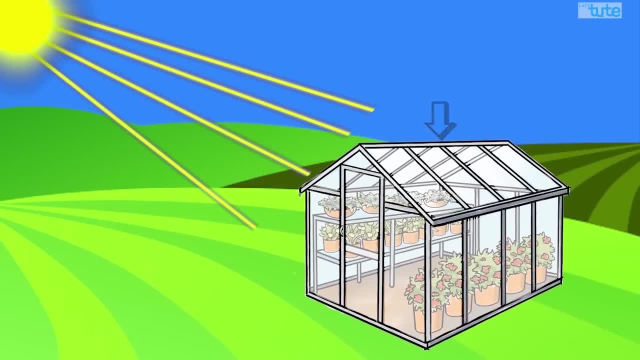 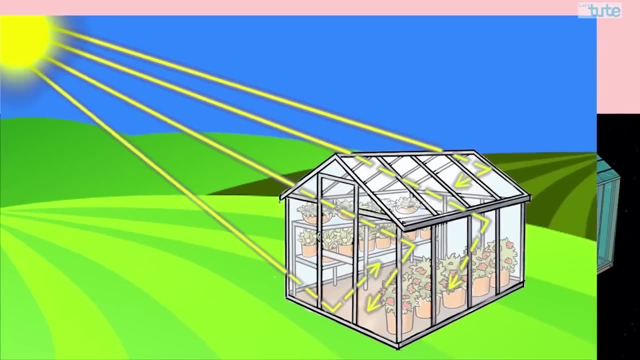 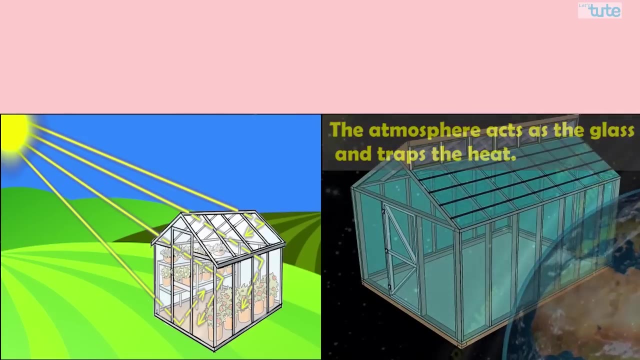 A greenhouse is a glass building in which plants that require protection from cold weather are kept. The glass cover helps to trap all the heat energy And keeps the inside environment warm. Now consider our planet earth. The atmosphere acts as the glass and traps the heat. 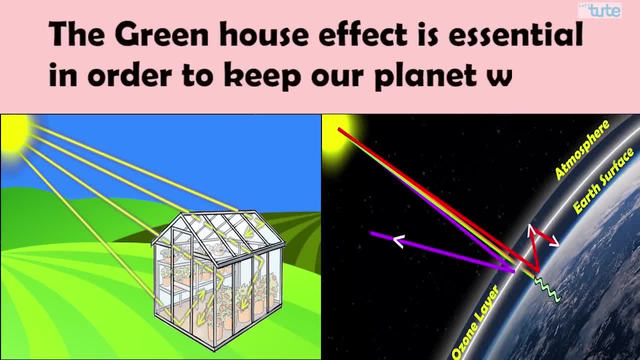 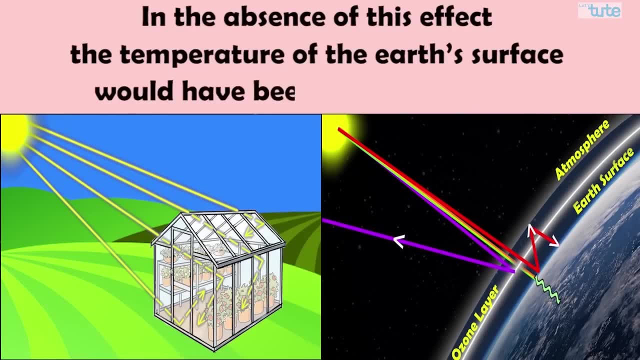 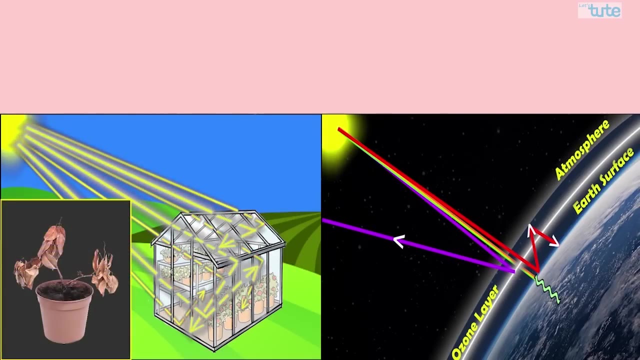 The greenhouse effect is essential in order to keep our planet warm. In the absence of this effect, the temperature of the earth's surface would have been minus 20 to minus 40 degrees celsius. But too much of something is possible. If the plants in the greenhouse receive excess heat, it would burn. 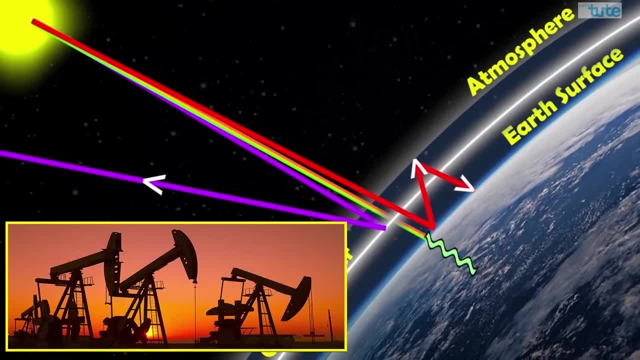 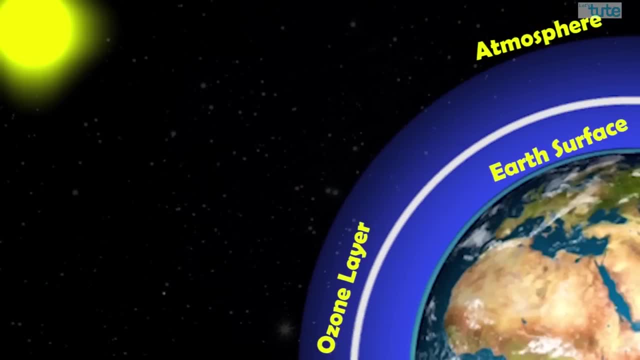 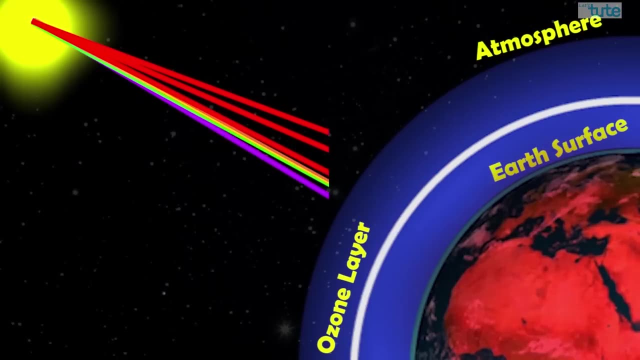 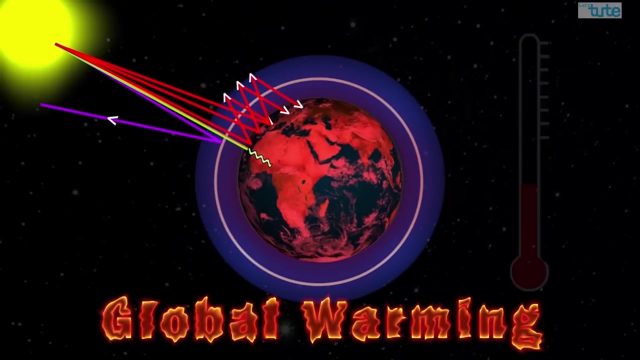 And if we consider planet earth, over the last two centuries, human activities have changed the earth's atmosphere in a dramatic way. The amount of greenhouse gases have increased and are still increasing. They trap too much heat, And this excess of greenhouse effect results in global warming. 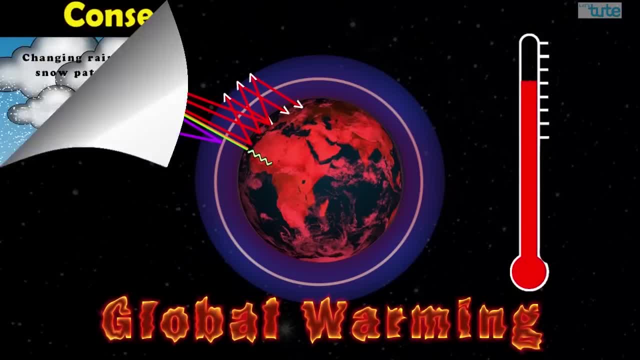 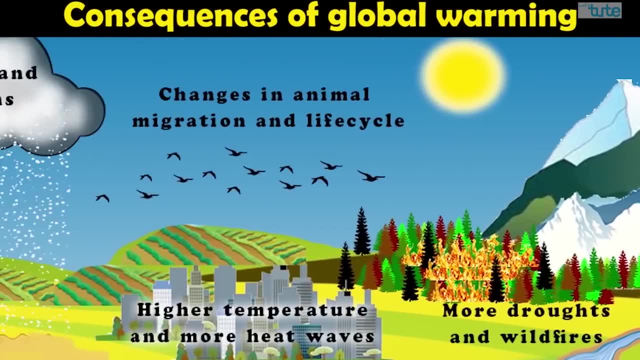 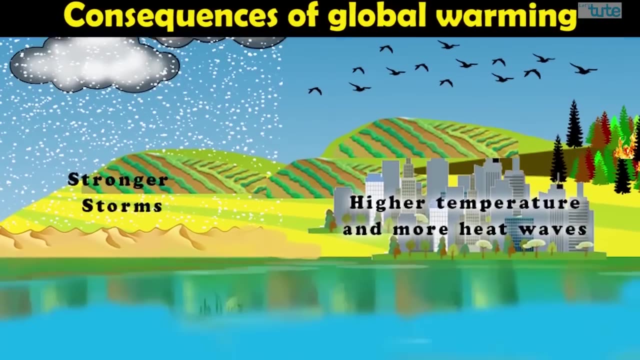 Which is an increase in the earth's average temperature. Consequences of global warming are enormous. Its effects are not limited to one country, but it would affect the entire planet, Knowing the fact that global warming exists and human-made carbon dioxide emissions have caused it.